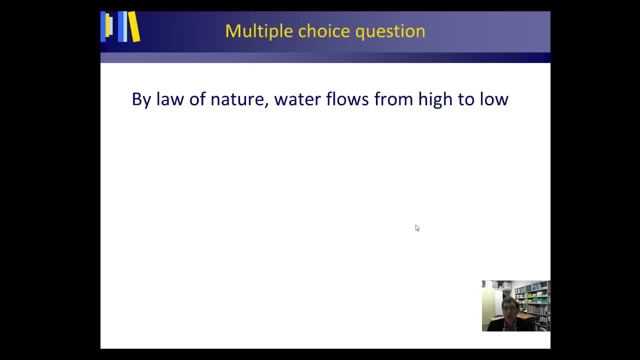 A multiple choice question. By law of nature, water flows from high to low Elevation. Is that the right answer? or is the right answer? By law of nature, water flows from high to low Energy. Or does it, by law of nature, flow from high to low? 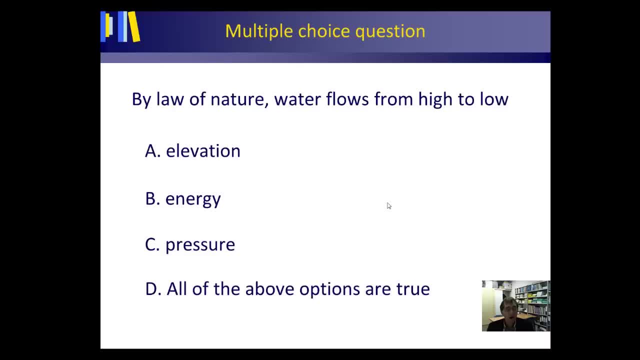 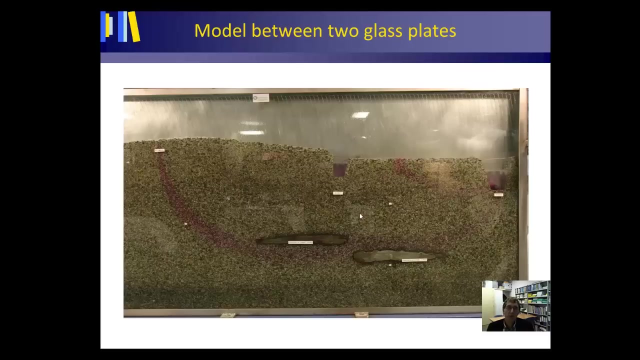 Water pressure Pressure, Or are all of the above options true? Think about this. There's only one right answer. What is the right answer? What do you think now And what do you think after you've seen this video lecture? Let's move to this model between two glass plates. 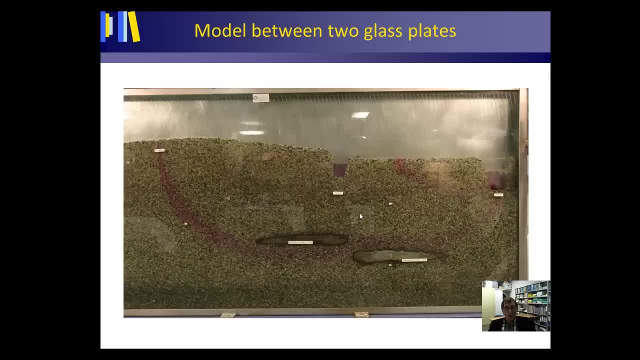 This is a model that we used during the open days of the Bachelor Institute of Earth Sciences here at Utrecht University. We have a model between two glass plates. This is the glass plate in front and there's five centimetres further down. There is another glass plate about five centimetres apart. 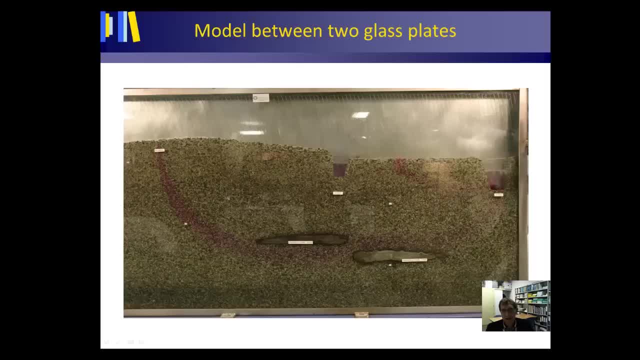 This is about 75 centimetres high. This is one and a half metres wide And, in actual fact, this is a replica of the subsoil, being 80 metres high and 13 kilometres wide, So there is a pronounced exaggeration of the vertical in respect to the horizontal. 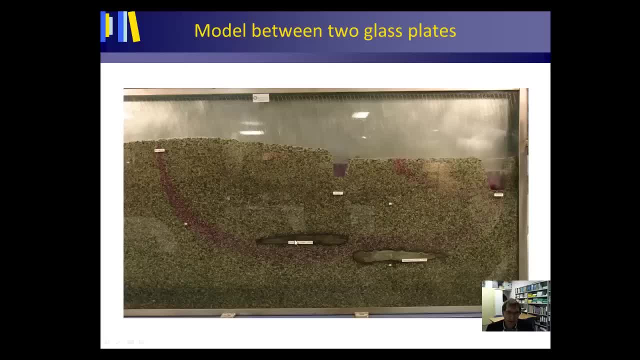 We see gravel here And we have sand there And in the real world this is sand And this will be clay. We have a higher part of the landscape here And here we have the flatter, polder part of the landscape. 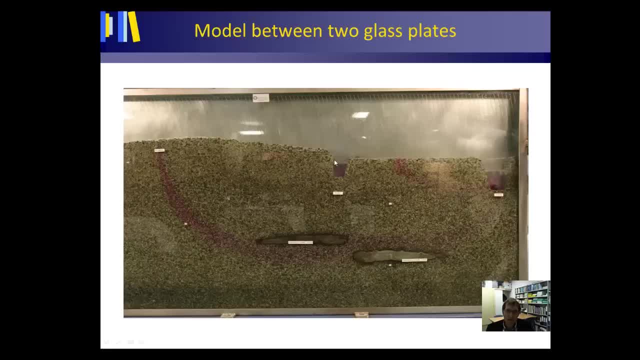 It's raining. Water is moving out of the model in this ditch And water is moving out of the model in this river. The water table is approximately like this. Of course, it coincides with the surface water level here And also here we have the water table like this: 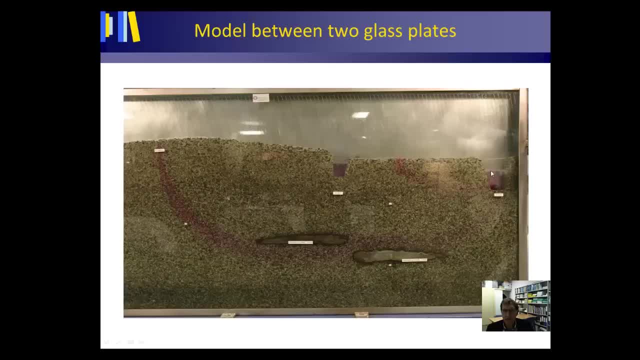 And it coincides with your surface water level. here, From the back of the panel, a colouring dye is injected into the system And this enables us to follow the pathway that the groundwater flow takes. And we see that groundwater flow from here flows in this manner, through these two clay lenses. 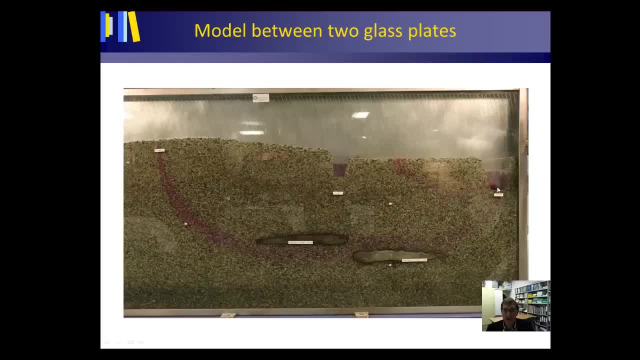 and then flows into the river. We call this a sub-regional or a regional flow line, And here we have a more local flow line And we can also see the movement of the water. So what do we see? We see that water is flowing along curved pathways. 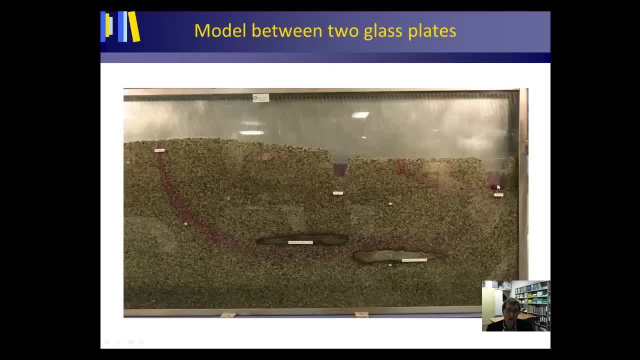 And we see that water can easily flow upward from a low to a high elevation. There's no problem in that, And also in reality, rivers are fed from below, And here we see, if we look here, we have a larger column of water. 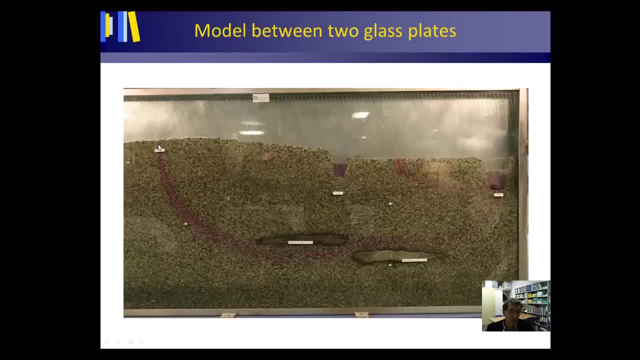 than if we look there, We have a shorter column of water. So water is flowing from a lower water pressure to a higher water pressure. It's flowing from a high to a low elevation, but from a lower to a higher water pressure, And here water is flowing from a higher to a lower water pressure, but from a lower to a higher elevation. So water can flow from high to low elevation, from low to high elevation, or from high to low water pressure and from low to high water pressure. There's no problem there. 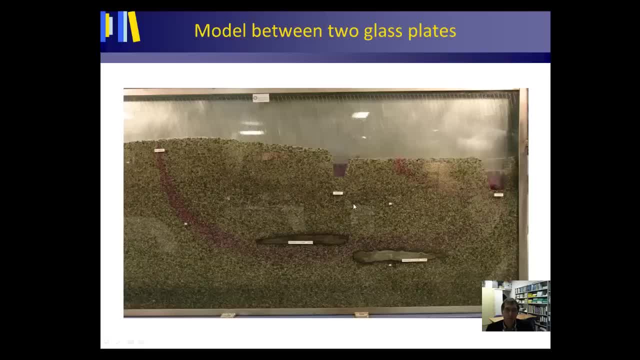 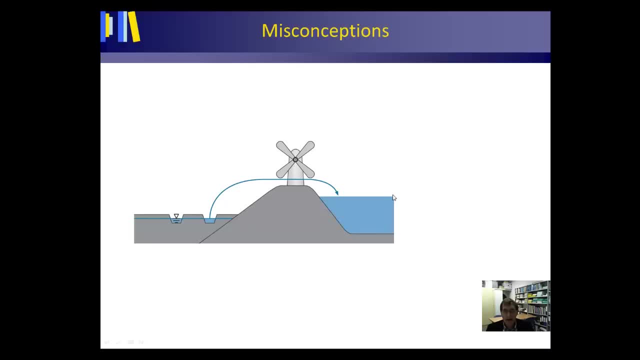 So what, then, makes water flow? Well, of course, this is a picture showing you the polder landscape again, Here we have a higher water pressure, to which the water from the polder is pumped, And if we would not do that, water would start to rise. 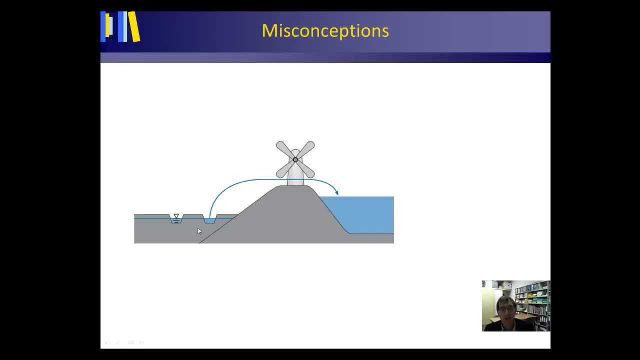 thus flow from a low to a high elevation. So we already knew that water can flow from a low to a high elevation. In actual fact, you already knew that water does not necessarily, by law of nature, need to flow from high to low water pressure. 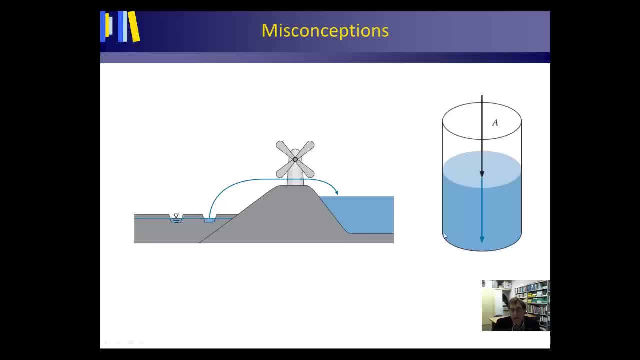 because if you look at the water in this cylinder, the higher water pressure is here at the bottom and the lower water pressure is here at the interface of the water with the air above. The water is at a standstill in this model. It does not by law of nature. 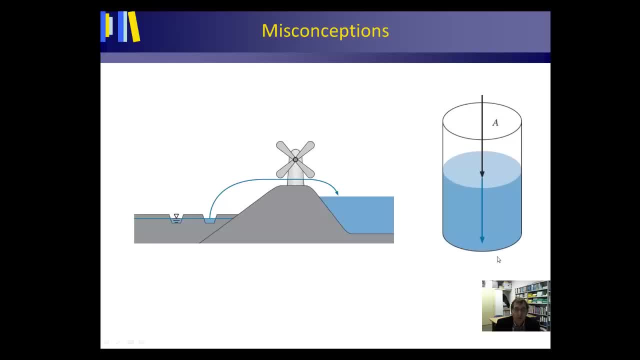 flow from a higher water pressure to a lower water pressure. So now we already know that two of the options in the multiple choice question- water flows from high to low elevation and water flows from high to low water pressure- are not true Water flows from high to low energy. 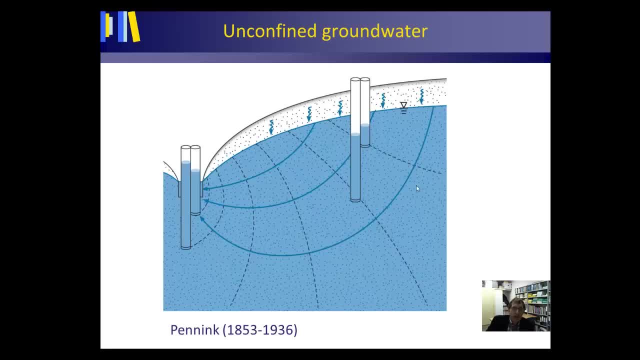 And we can very simply measure that energy using a piezometer, a steighoogtebuis. So your hydraulic head, if we take this as a reference level, is simply this height which I am indicating now, Your total energy here. 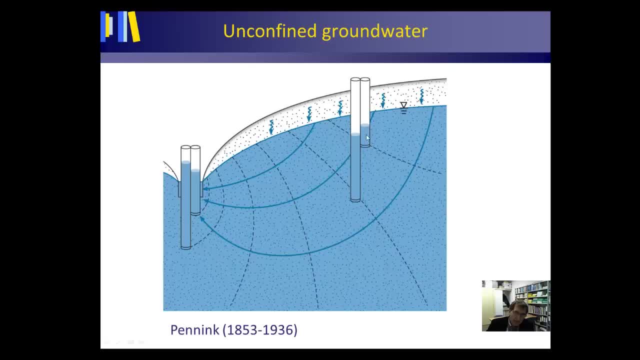 your hydraulic head is this height, So we have a higher hydraulic energy, a higher total energy here than there, meaning that water is flowing downwards. Here we have the river. Of course, this was the upper part of your landscape, with here your water table. 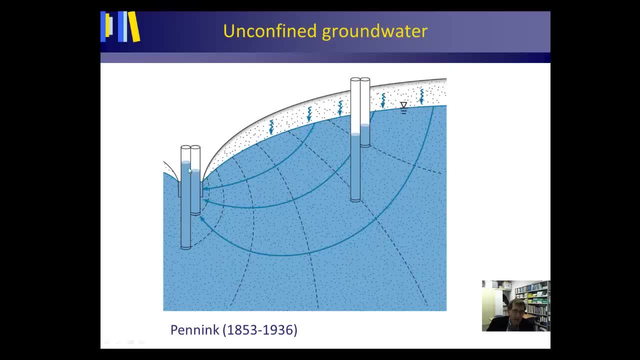 Water table coincides with your surface water level here. And if we install two piezometer tubes here also, of course you must take care that there is no leakage from the river water. We can estimate or we can actually determine the hydraulic head here. 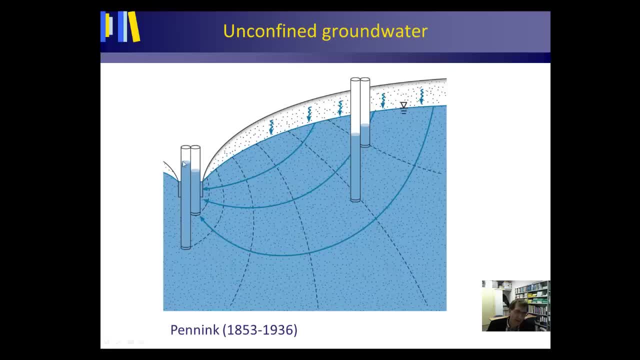 simply as the height to which the water rises again in this tube in respect to this reference level. So this is the hydraulic head at this location and this is your hydraulic head at that location, My hydraulic head here, deeper down in the subsurface. 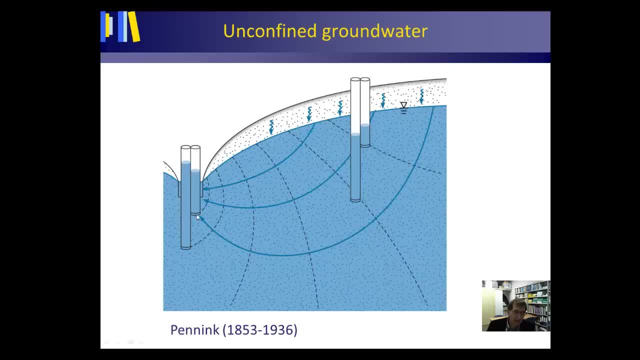 is higher than my hydraulic head here, higher up in the subsurface, meaning that water is flowing upward. If we were to install more piezometers, we could establish this figure of streamlines where water is flowing here it's recharging. 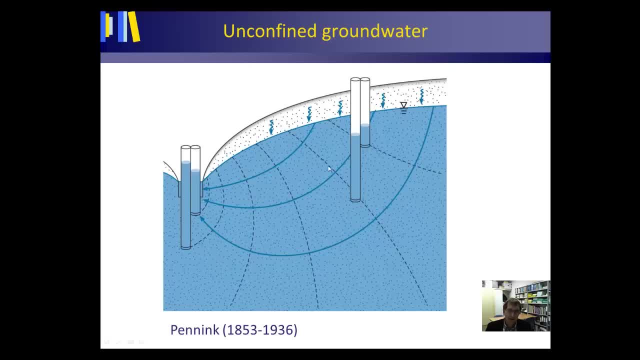 and here it's discharging into the river And, in actual fact, these broken lines are lines of equal energy, of equal hydraulic head. So this is a higher hydraulic head, this is a lower hydraulic head and this is an even lower hydraulic head than here. 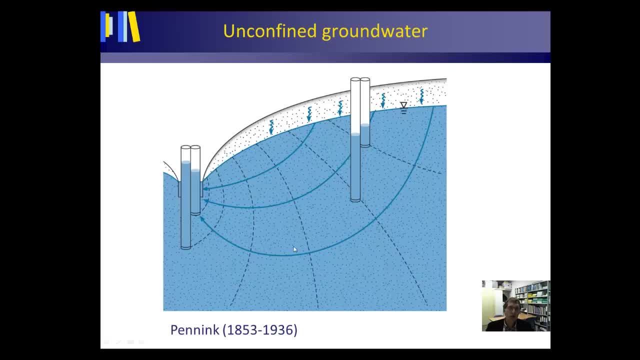 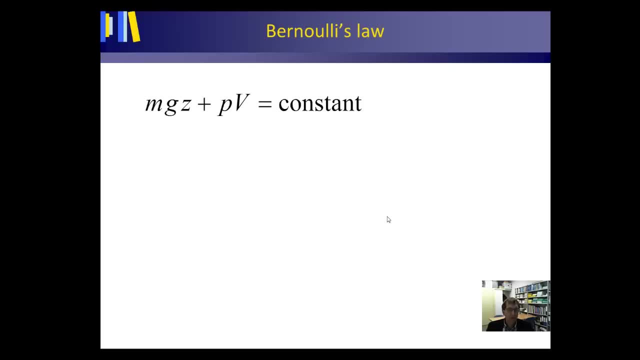 Water is always flowing from a higher to a lower energy or from a high to a low hydraulic head. If we look at Bernoulli's law, Bernoulli's law states that if we have, if there is no loss of mechanical energy. 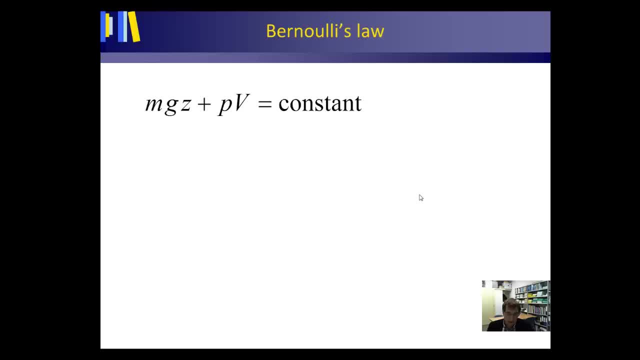 due to friction, and also if we take water as incompressible, then for steady groundwater flow. Bernoulli's law states that the sum of certain energy terms is constant. In actual fact, there are three interchangeable energy terms. One is kinetic energy. 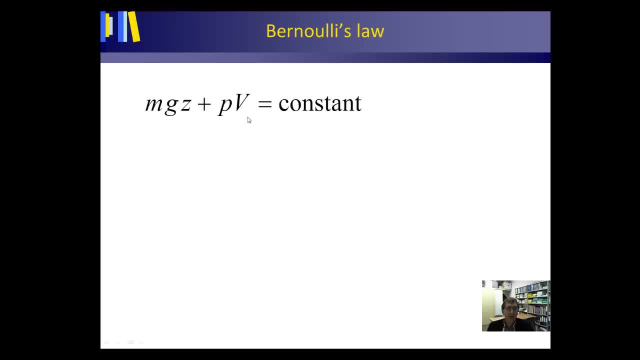 which has to do with the velocity of the groundwater. I can already tell you that the velocity of groundwater is very low. Groundwater flows very, very slowly, So we can forget about that term in Bernoulli's law. So you don't see it here. 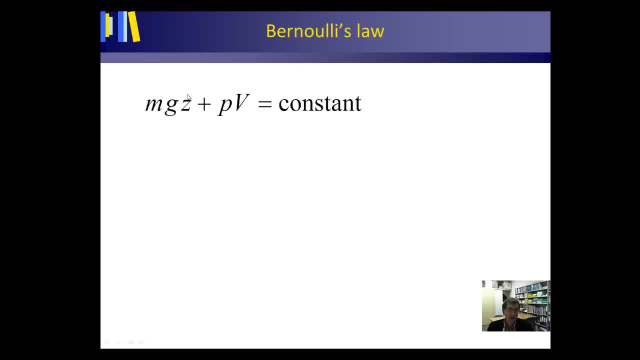 Instead, you only see here potential energy and you see here pressure energy. Of course. m is the mass of the water in kilogram, G is the acceleration due to gravity, which is approximately 10 meters per square second, And z is the height or the altitude. 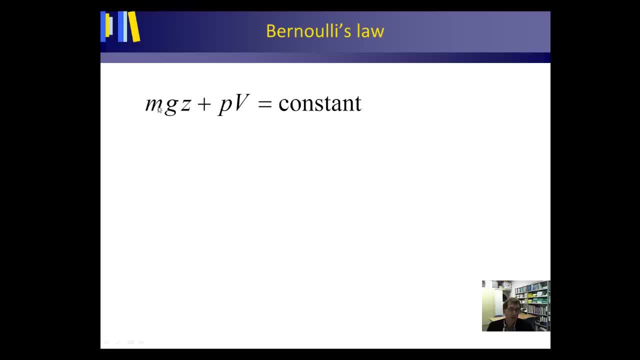 above reference level. Kilograms times meter per squared. second times meters gives you joule as an energy term here. Here we have the pressure. This is your pressure energy. P is pressure in Newton per square meter And V is your volume of your water. 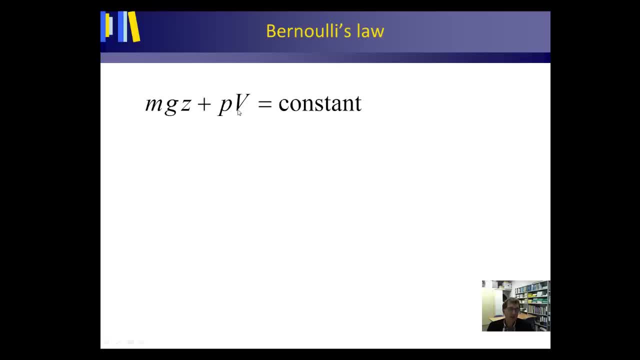 in cubic meter. So Newton per square meters times cubic meters gives you Newton meters, which is also joule. So this is constant, as I just told you, And we can simplify the equation. We can divide all terms to the left and the right. 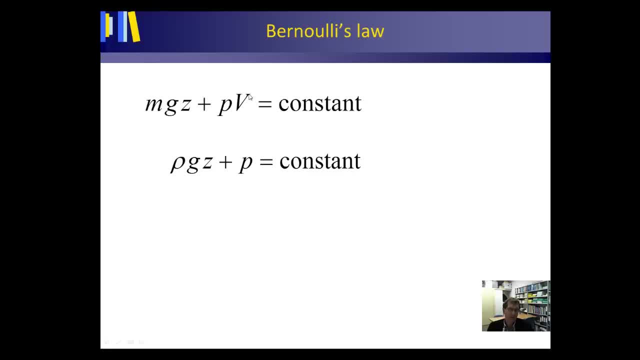 of the equal sign by the volume of the water. So you could also say we're looking at a certain volume in the subsoil. Then mass of course becomes density, So kilogram becomes kilogram per cubic meter. These of course stay the same. 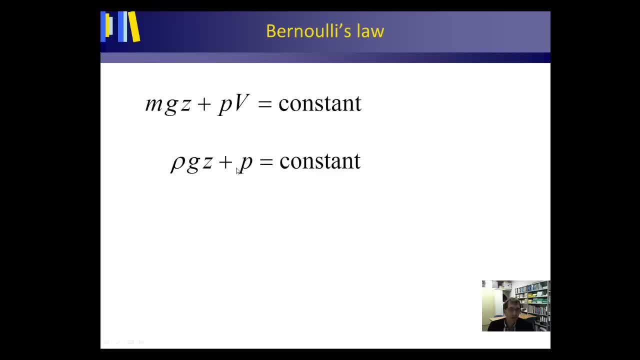 And if we divide by volume, your PV terms of course, becomes P, And this is also constant. In actual fact, this constant now divided by V, by the volume, We can simplify it even further. What we can do is we can divide by density. 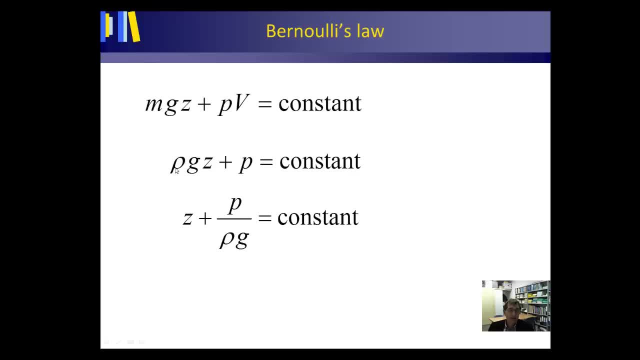 because fresh groundwater has a constant density of a thousand kilogram per cubic meters And we can divide by the acceleration due to gravity, Because that's at a certain location is also a constant. And if we do that, if we divide, rho g z. 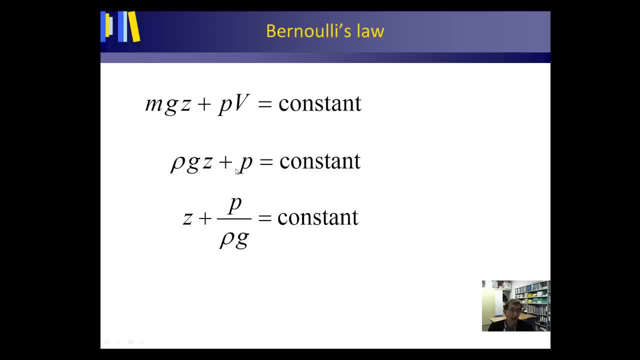 by rho g, of course we get C. And if we divide P by rho g, z, this is what we get. And also these terms added together are constant And of course what we see now this term is in joule, Also this one, of course. 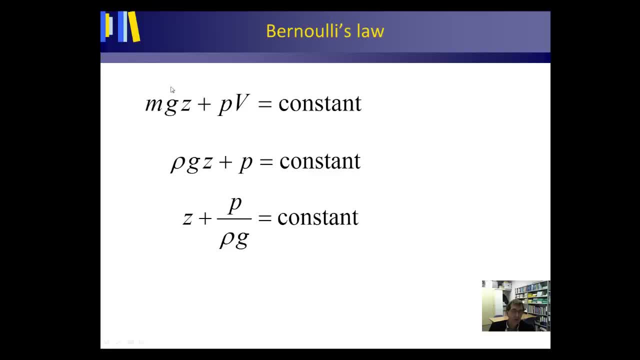 But now we find here the terms in meters. So we have come from energy terms in joule to energy terms expressed as a length unit. And what's the connection with the piezometer tube? Well, let's tell you first about this Also, the connection will become clear. 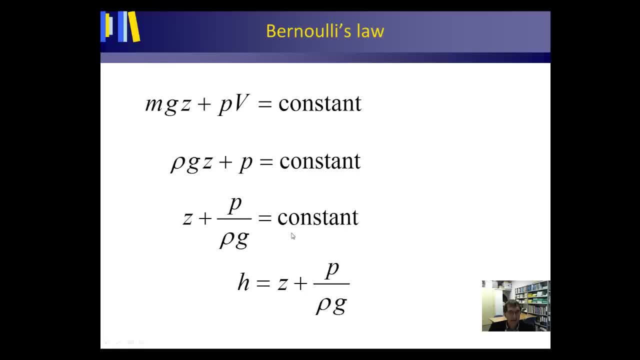 This constant. we call it the hydraulic head. stijghoogte, The z we call elevation head, plaatshoogte in Dutch, And P divided by rho. g we call it pressure head or drukhoogte in Dutch. 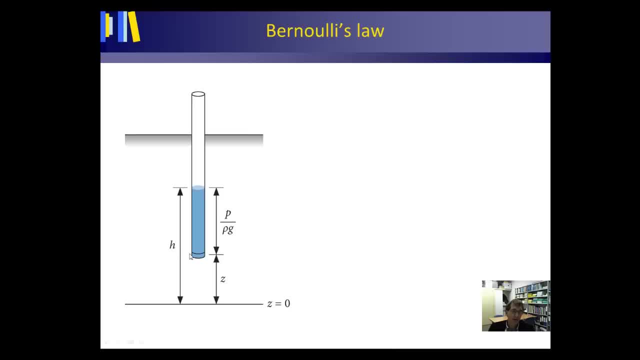 So if we have a piezometer tube- and I already explained water can only flow in through the bottom of the tube, through the screen- Then z is simply the altitude above your reference level. P divided by rho, g is simply the water pressure here at this location. 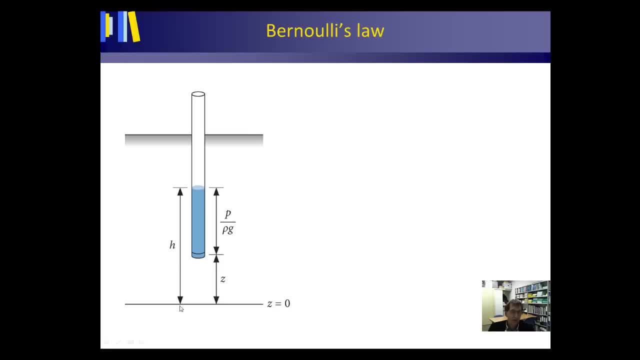 And if we add z plus P divided by rho g, together we get H, the hydraulic head. So hydraulic head equals elevation head plus pressure head, And the Dutch word hydraulic head stijghoogte, elevation head plaatshoogte and pressure head drukhoogte. 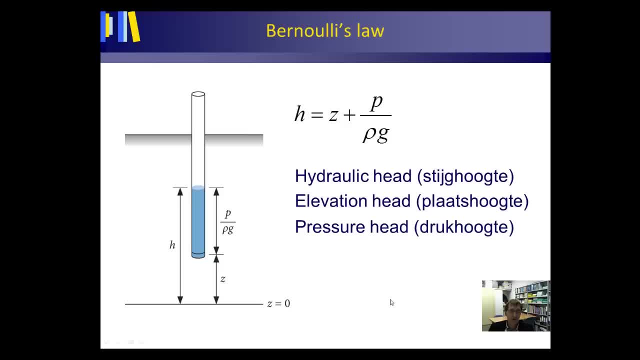 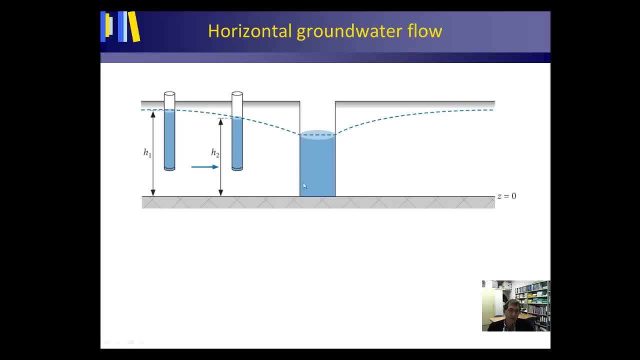 And again piezometer tube. in Dutch we call that a stijghoogtebuis, So if you have horizontal groundwater flow, this is a ditch. this is a cross section through the landscape. of course, We have installed two piezometer tubes. 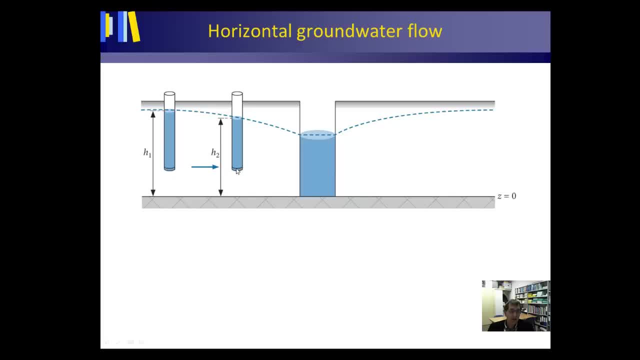 with their screens at the same altitude above this reference level, we find that the water flows to a higher level in this tube in comparison to this tube. So here we have a higher hydraulic head, a higher total energy than there, meaning that water is flowing in the direction. 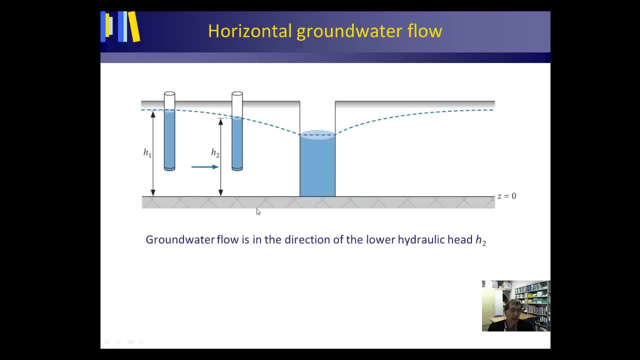 of the lower hydraulic head, H2, and that, in actual fact, come back to the earlier multiple choice question. the right answer must be that water flow is from a high to a low energy, from a high to a low hydraulic head. This, of course, is horizontal groundwater flow. 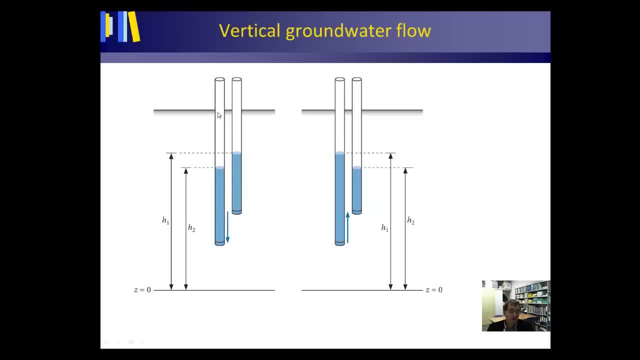 but if you were to install two piezometers close together in the subsoil, one with its screen at deeper down in the subsoil and one with the screen not so deep down in the subsoil, then we could simply establish: water is always. 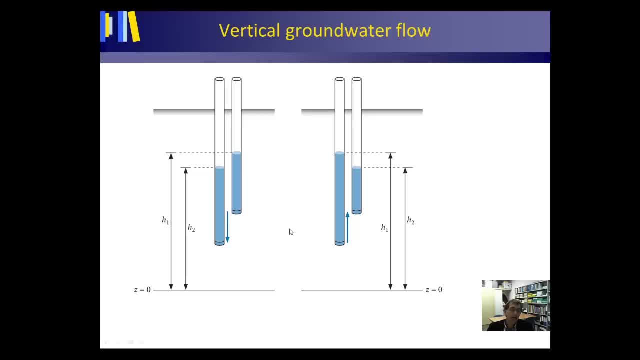 flowing from a high to a lower hydraulic head, the direction of the water flow. Well, here we find, at a higher location in the subsoil a higher hydraulic head H1 than deeper down. Here we have a hydraulic head H2, meaning that water is flowing. 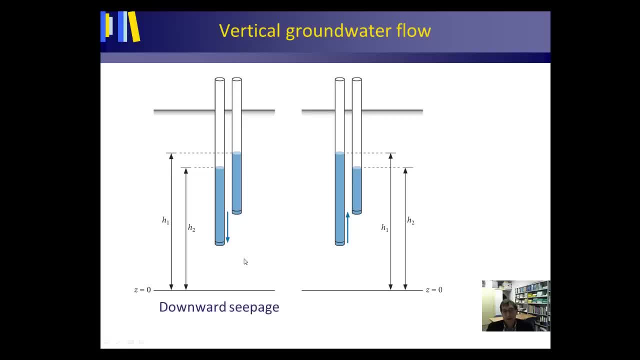 downward, downward seepage, and with a kind of old fashioned Dutch term, we call that wegzeiging. Here we have the opposite. here we have water which is upward. and why is that? It's simply because we are measuring a higher hydraulic head here. 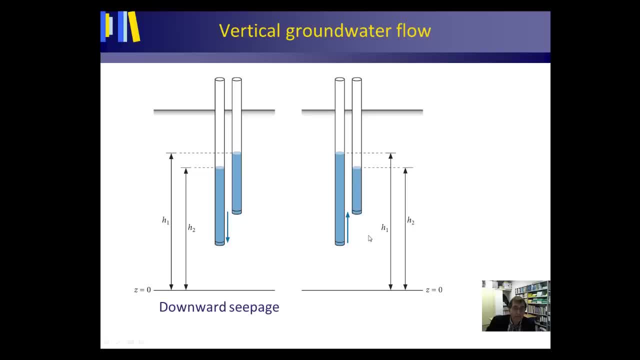 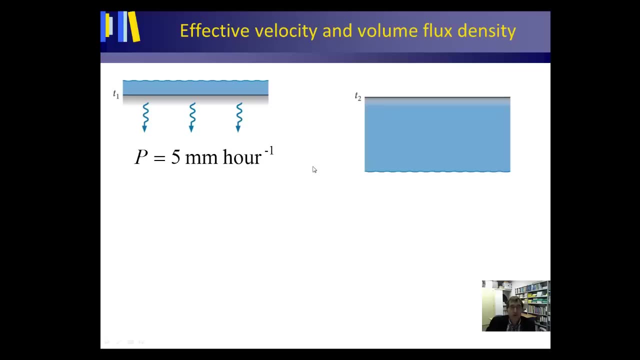 a higher total energy here than we are measuring here, and in Dutch we call this sorry, in English we call this upward seepage and in Dutch we call this kvel. Let's do a little mind experiment to show you the difference between velocity and volume flux. 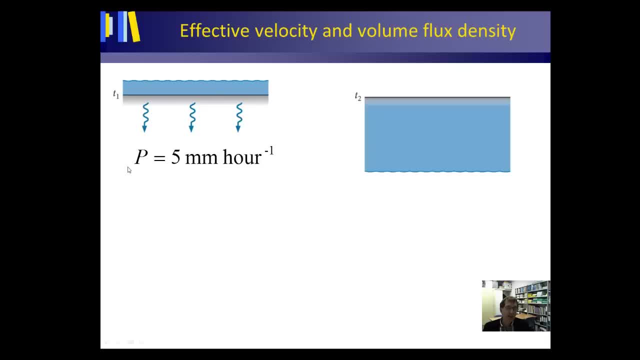 density. It's raining, and let's imagine that it's raining on a soil which is 100% dry. So we have 5 mm of rainfall in an hour and you can think of that 5 mm of rainfall as a layer on top of your. 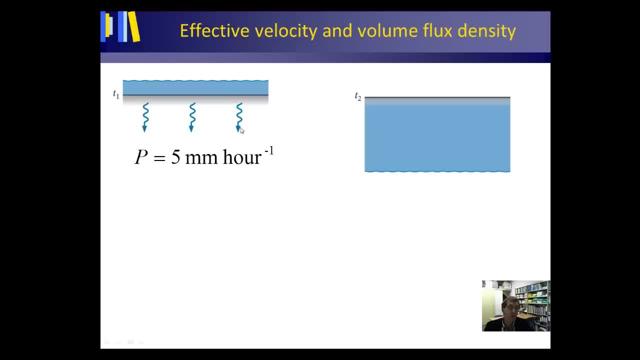 land surface, which is infiltrating into the pore space of your subsoil. The question is: how deep will the water infiltrate into this 100% dry soil? Well, let me ask you: will it be 5 mm, or will it be less, or will it be more than 5 mm? 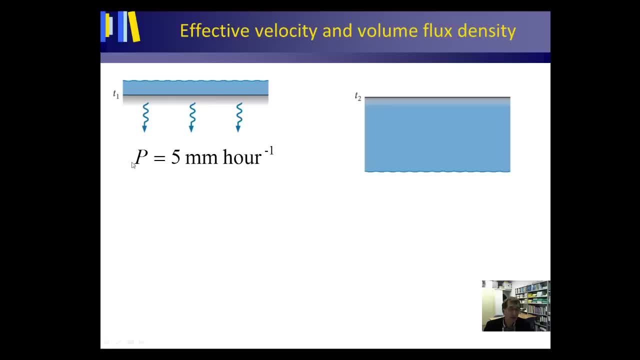 Of course it has to be more than 5 mm, because your subsoil is made up of pores and in between these pores, these minute holes in the soil, we have solid substances and we call that the matrix. So let's imagine that water infiltrates to a depth of. 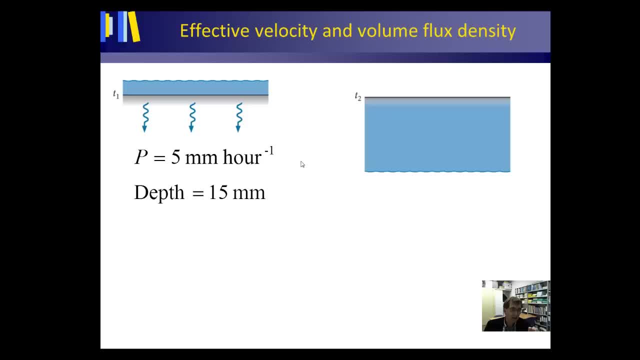 15 mm. You could first of all ask yourself: how much volume of pores do I have in the subsurface as compared to the total subsurface? Well, that must be 1 third If I have 5 mm of rainfall and this infiltrates into the soil. 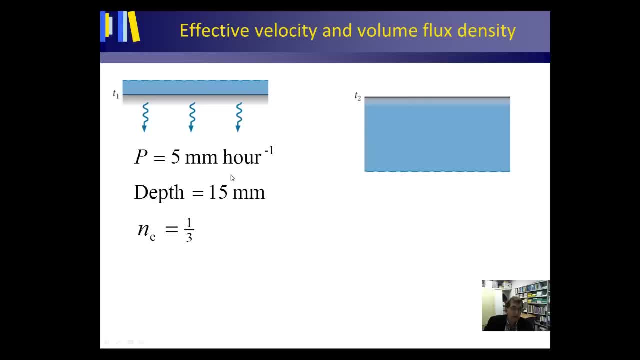 and it attains a depth of 15 mm, then apparently I have a pore space of 33% or 1 third and water can only go into these pores. water does not flow into the solid soil matrix. We call this the effective porosity. 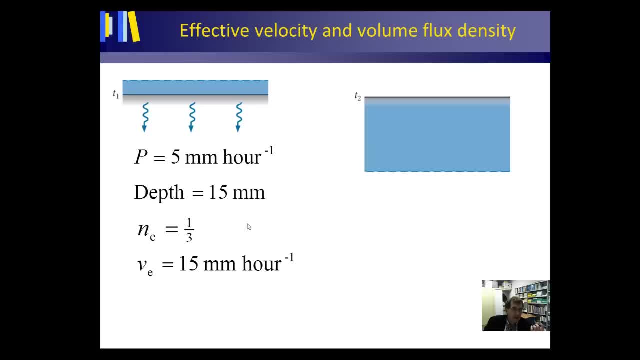 And of course water reaches a depth of 50 mm. so the velocity of the water in this 1 hour is 15 mm per hour. But we can also say that 50 mm per hour is infiltrating into the soil, and this we call the volume flux. 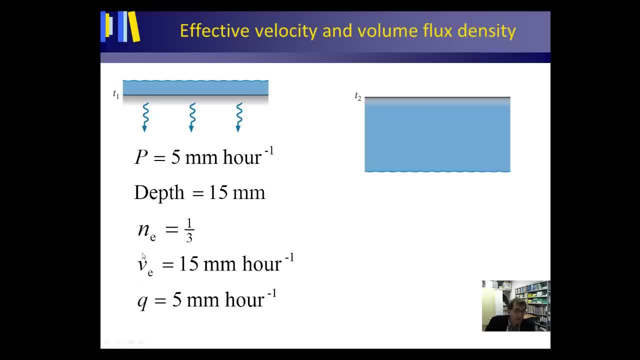 density. So your effective groundwater velocity, or your effective water velocity here, is 50 mm per hour and your volume flux density is 5 mm per hour. So this is an essential difference between effective velocity and volume flux density, both measured in, for instance, mm per hour, or it could be. 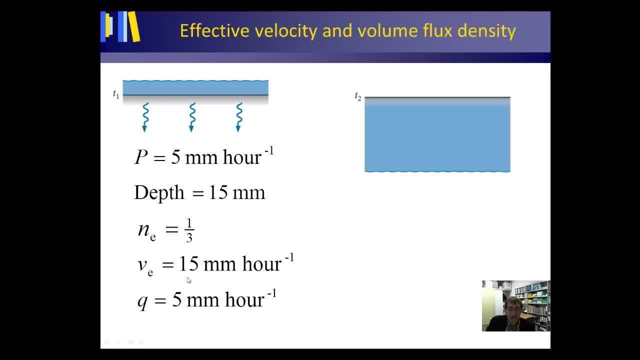 mm per day. but you see that the numbers are different. And what's the relation? Well, you can already see it: if your effective velocity is 15 and your effective porosity is 1 third, then your volume flux density is 5 mm per hour. 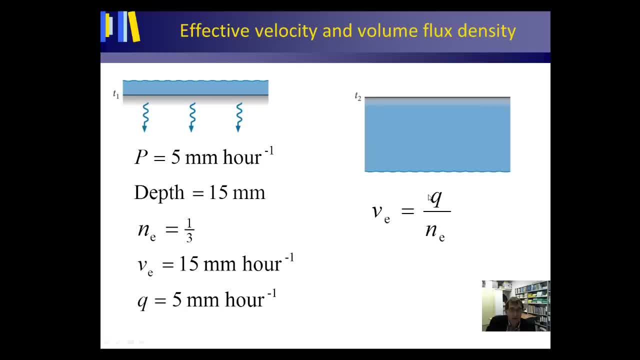 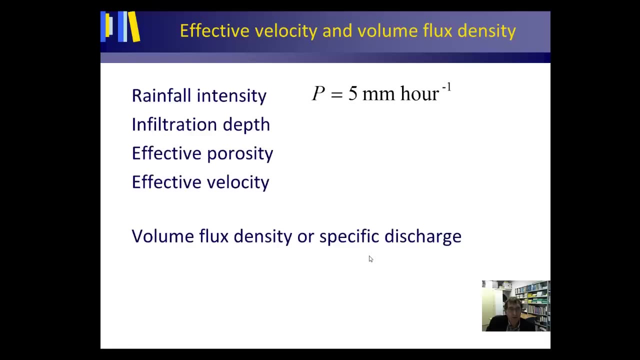 or more usually, what we do in hydrology is determine the volume, flux density, and if you divide that by your effective porosity, you get your effective velocity. So, in summary, rainfall intensity of 5 mm per hour on a 100% dry soil. let's imagine that it reaches. 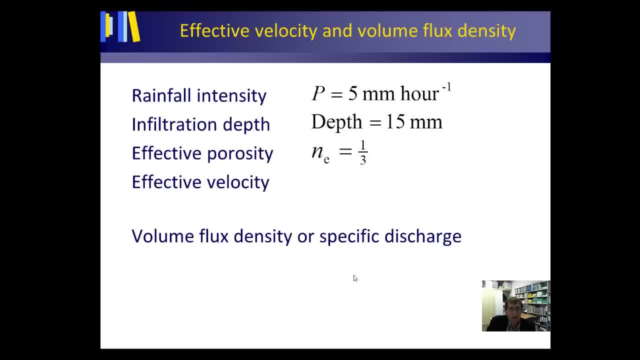 the water reaches a depth of 50 mm, that means that your pore space is 1 third of your total soil. so you have 1 third of your soil. Your effective porosity is 50 mm per hour, de werkelijke snelheid, we would say in Dutch. 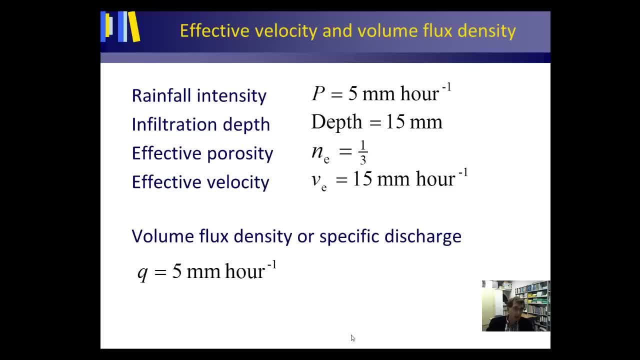 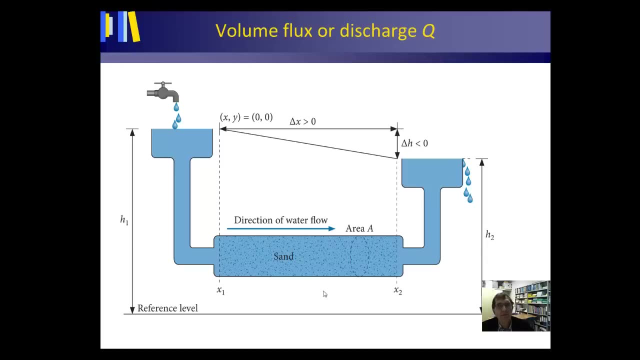 and your volume, flux, density or specific discharge. je volumestroomdichtheid of specifieke afvoer is 5 mm per hour and Ve equals Q divided by Ne. Let's have a look at this experiment by Darcy. We have a sand filled cylinder. 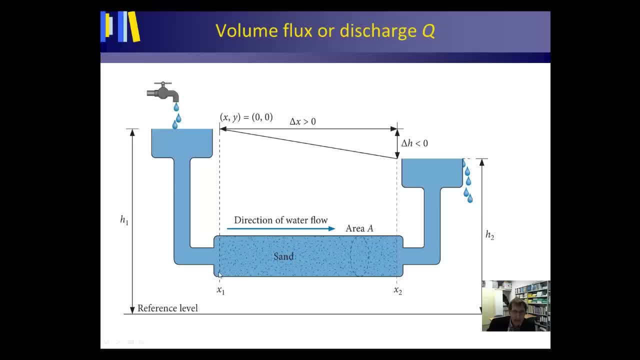 so this is the cylinder. here we have the sand and here we have a tube and water rises to this level in the tube and at the right hand side water is leaving the tube again and is dripping out, so we can collect the water here and determine the amount. 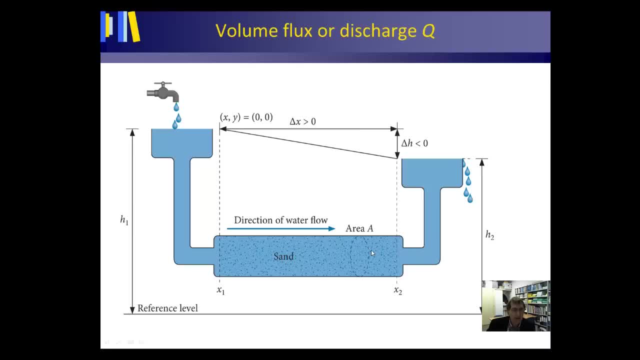 or volume of water which is passing through the sand column. of course, this is a screen which keeps the sand in place but lets the water flow in, and the same screen we have here, and here we see the area of your cylinder, which is also the area perpendicular to your 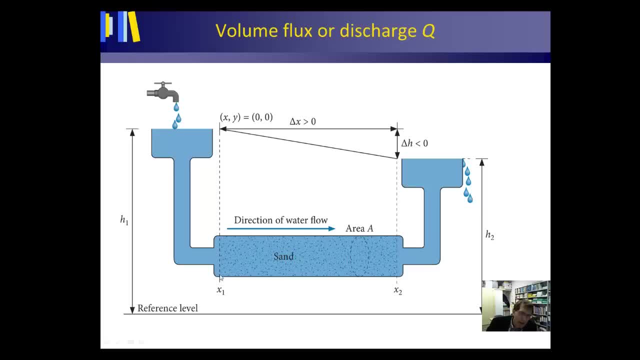 water flow. Well, if we were to look at this screen and establish the hydraulic head here, for instance in the mid part here, this would be your elevation head and, of course, this part would be your pressure head, and then elevation head plus pressure head gives you hydraulic head. 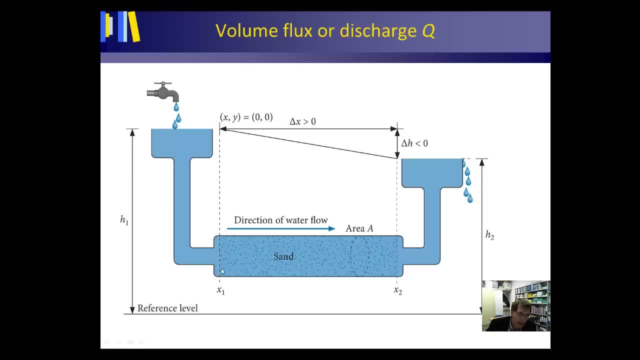 well, everywhere along this screen, whether I am looking here or here, or here or here, the hydraulic head is the same. so I have a fixed hydraulic head of H1 here. Similarly, I have a fixed hydraulic head but a lower hydraulic head- H2- here. so water is flowing from. 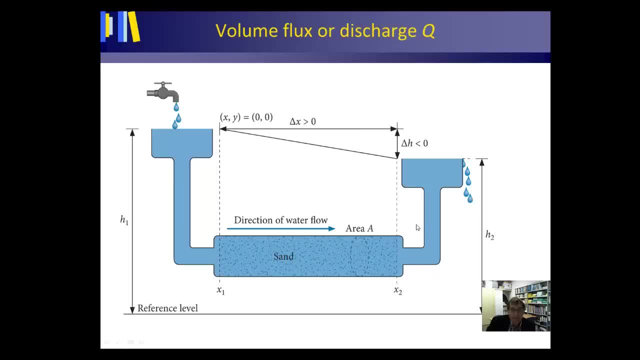 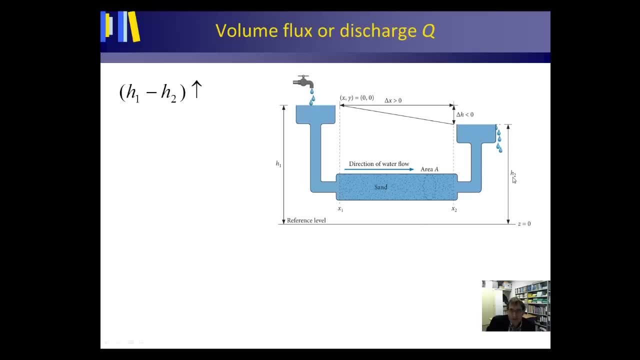 left to right through this system. well, lets do a thought experiment. what would happen if the difference between H1 hydraulic head here and the hydraulic head at this screen, if I would enlarge it so I could rise this tube or I could lower this end, lower this tube. 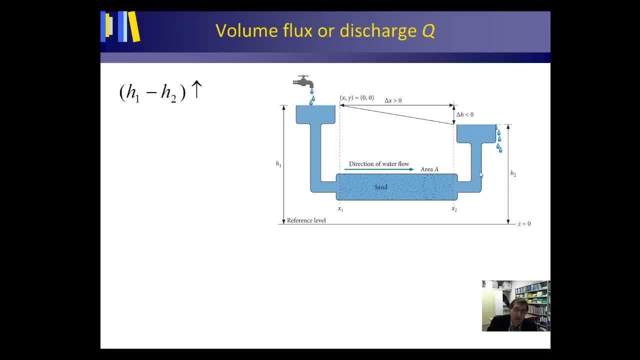 well, intuitively, you think that the discharge or the volume flux of the would of course get bigger. so H1 minus H2, when that becomes larger, Q will become larger. what will happen when the distance X2 minus X1 diminishes? well, of course, the porous medium which is 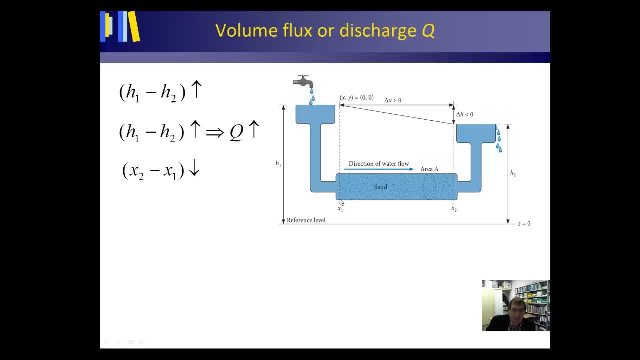 resisting the water flow gets smaller, so it is easier for water to pass through and your discharge would increase. what would happen if we would enlarge the area A perpendicular to your flow? Well, of course, if you enlarge this area A, you also enlarge the area of the porous. 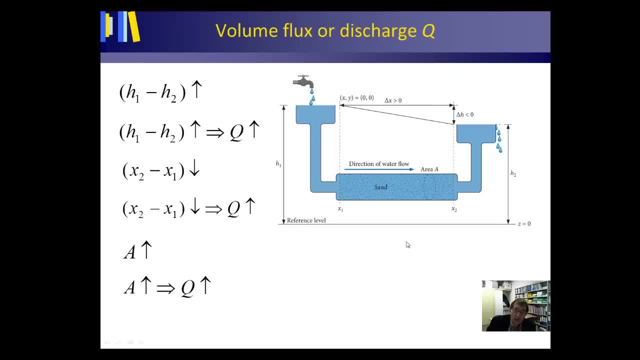 within this area A and your Q will become larger. so, interestingly, this area, water is only flowing through the porous and not through the solid substances. in this instance, when we have sand, we have sand grains and water is only flowing in between sand grains. we can already 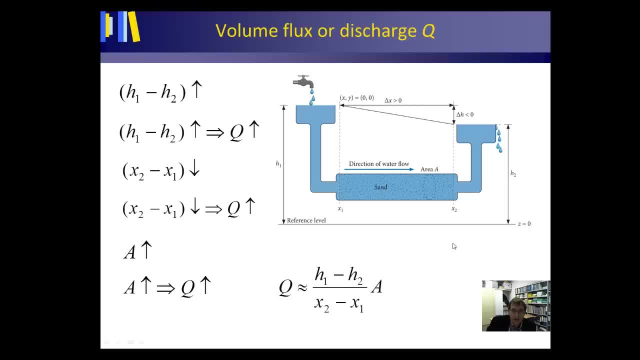 establish part of Darcy's law by this, because we can see that your volume flux, your discharge, is linearly related with the difference H1 minus H2 of these two hydraulic heads. it is inversely and linearly, inversely linearly related with X2 minus. 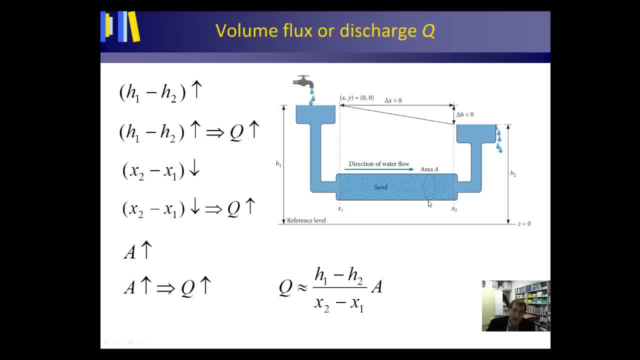 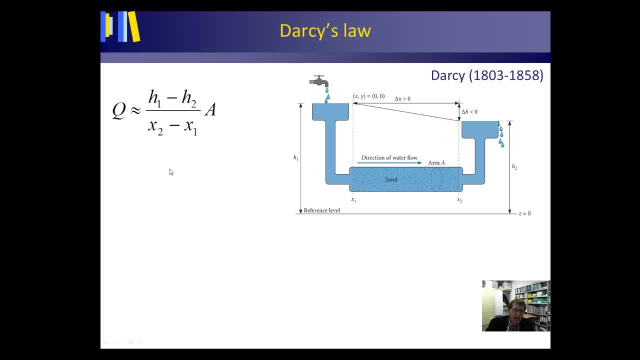 X1 and it is linearly related with the area A. so here we have it again, but we can already see. ok, this is not looking very neat, because here I have a term with 2 minus a term with 1, and here it is the other way around. 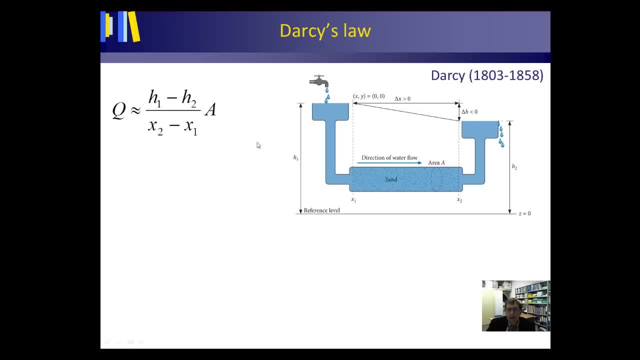 so let's define the difference in hydraulic head as the hydraulic head to which the water flows minus the hydraulic head from which the water flow dispatches, so through the porous water resisting medium, that is H2 minus H1. and then, of course, we can rewrite this part. 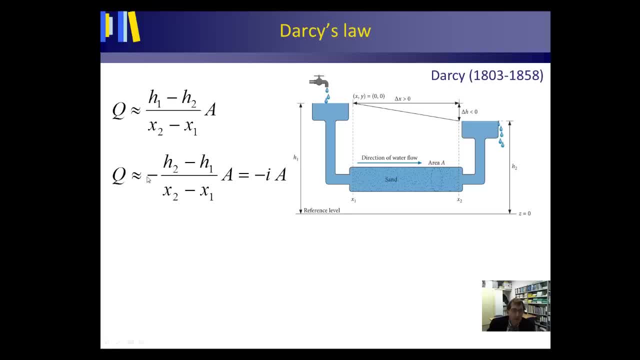 of the equation as Q being related to H2 minus H1 divided by X2 minus X1 times A, but now, of course, we have the minus sign inserted here. in actual fact, this term, your difference in hydraulic head divided by the difference in location, through which 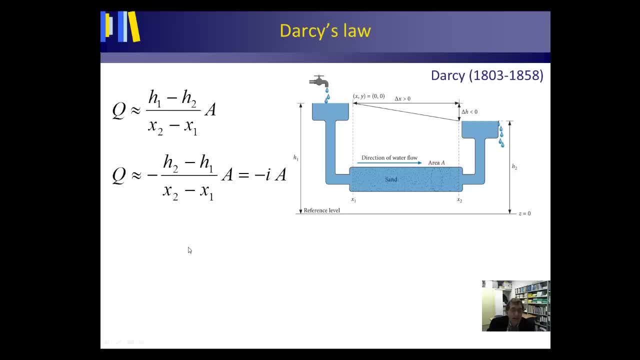 the difference in hydraulic head is attained. we call this the hydraulic gradient and we denote that with a small i. so Q equals minus the hydraulic gradient times this area perpendicular to your water flow, in actual fact this area A, you can look upon it as a kind of false area. 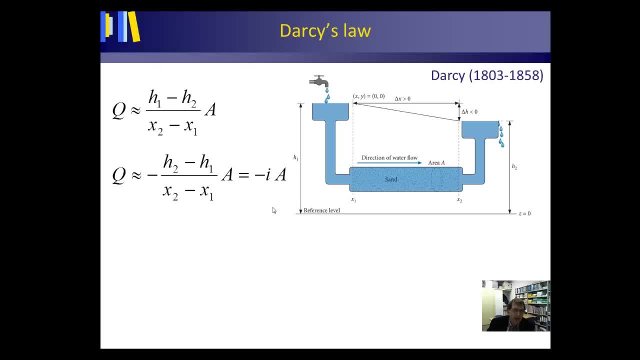 water is not flowing through the area in full, it is only flowing through the pore space in this area. well, you see here that we need another term. and why is that? it is because, if you look at this equation, this is in cubic meters per second, per day. 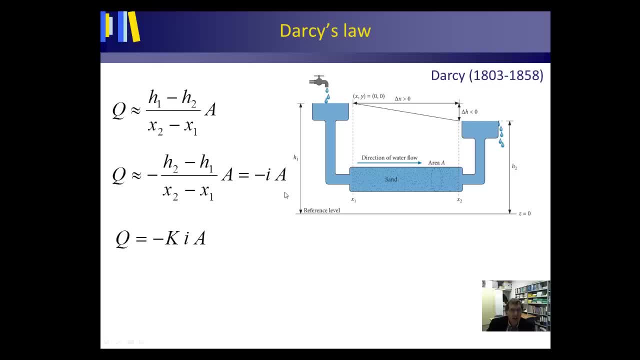 this is meters divided by meter, so that is dimensionless and of course, A is in square meters. so if we have square meters here and cubic meter per day there, we are still lacking a term meter per day, and that is this term K which is called the hydraulic. 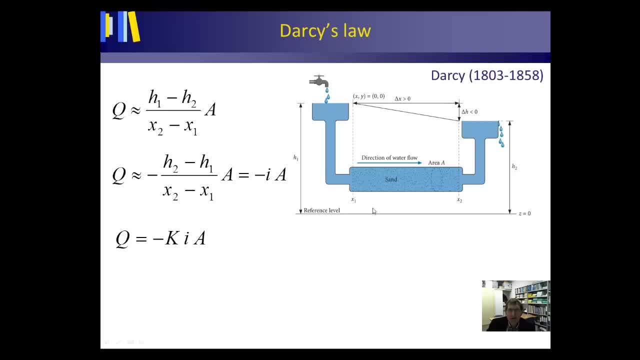 conductivity, and the hydraulic conductivity has to do with the material that we have placed in between these screens. if it is sand, or if it is loam, or if it is clay, etc. this will influence your water flow also. so K we call it the hydraulic conductivity, and it has a unit of 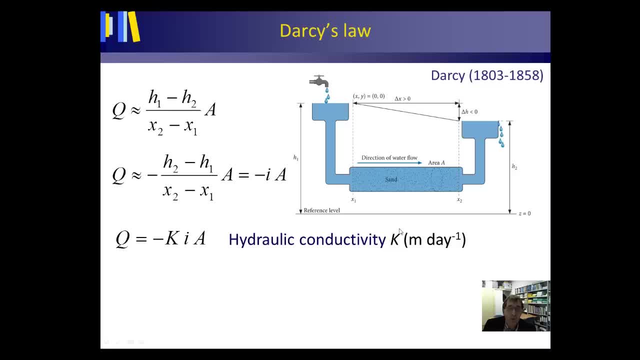 meter per day. in actual fact, K also has to do with properties of the water. is the water warmer or is it colder? it will mean that the density changes a little of the water. the viscosity of the water changes also, and this also influence water flow. all these 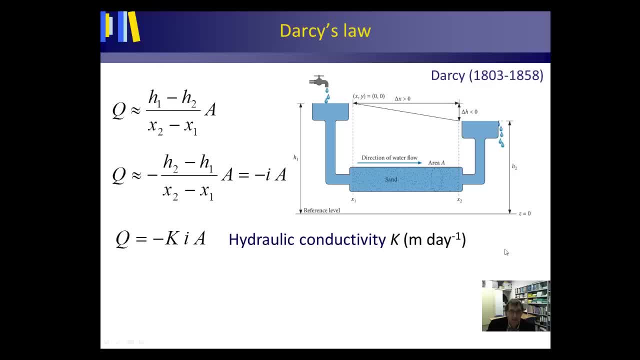 variables are kept structured in this, in this variable of hydraulic conductivity. so this is in actual fact already Darcy's law. but if you look in literature you usually find it expressed as small: q is minus K times your hydraulic gradient. and of course here already we recognize that this 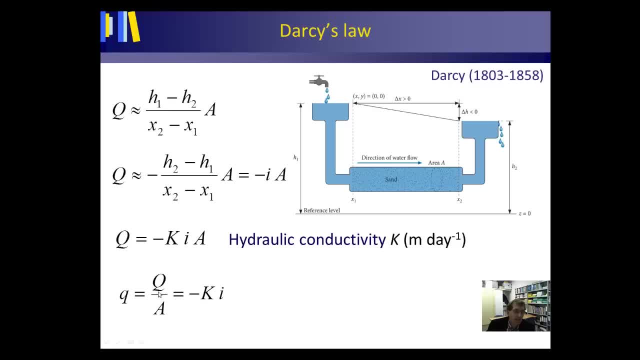 small. q must be your volume flux density, because it is your volume flux divided by an area A. but this area A is containing the solid substances and the pores, but water is only flowing through the pores and this means that this can never be a velocity but has to be a volume flux density. 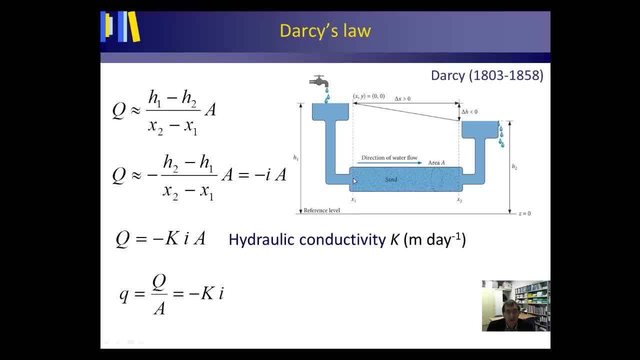 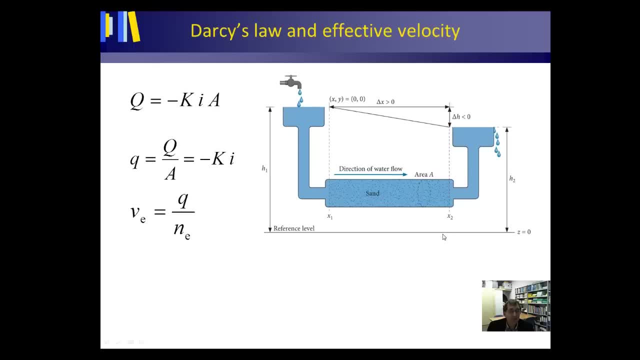 if I want to know the real groundwater velocity of water flowing from x1 to x2, of course I need to know the effective porosity. and here we have it: if you divide your volume flux density by your effective porosity, you will attain your effective velocity. 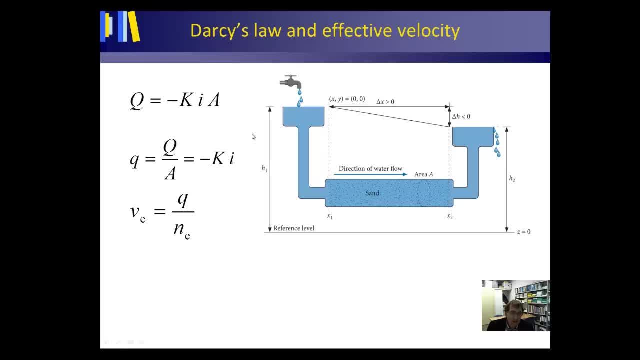 of your water flow. so we have Darcy equations in two forms here and we have this important equation and with this we can determine, for instance, if there was a pollution. here we can also determine the time it takes. if we know the groundwater velocity, we can determine the time. 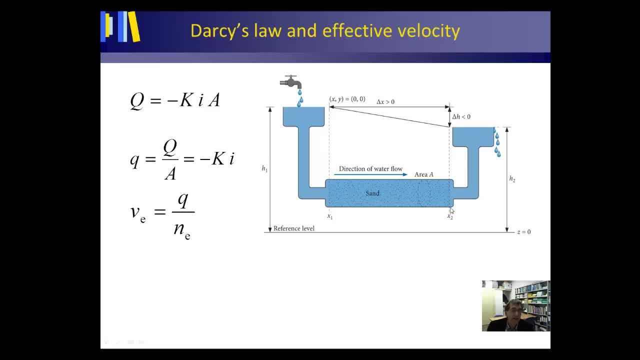 it takes to reach this end of your cylinder. so to put things, to summarize things, we have volume flux or discharge q in cubic meters per day, the volumenstrom of the afvoer in cubic meter per dag. we have volume flux, density or specific discharge small q in meters per day. 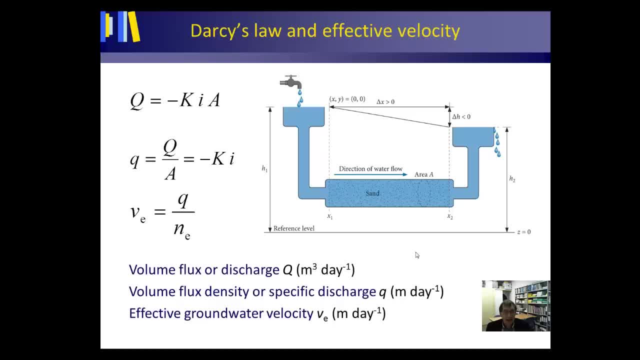 the volumenstromdichtheid of specifieke afvoer- kleine q in meter per dag. we have effective groundwater velocity also in meter per day, but this is the real velocity of your groundwater flow, the real velocity of your water flow. so if we come back to our 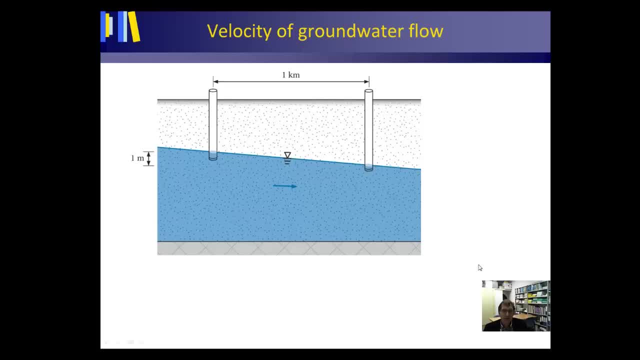 original problem. can we determine the velocity of the groundwater flow? yes, that's quite easy. let's imagine that this is a sand body, a sandy aquifer. then your k value will be in the order of 10 meters per day and your hydraulic gradient, when this is water, which? 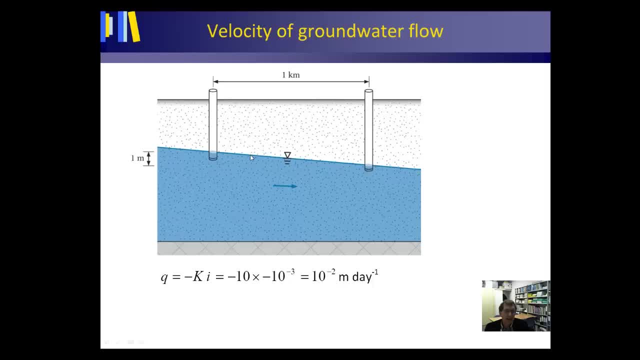 can flow freely when it's not confined in between two confining layers. but when the water table can establish itself freely, then you will find that the hydraulic gradient is approximately one meter per one kilometer. so that's one meter per thousand meter. so that's 10 to the minus. 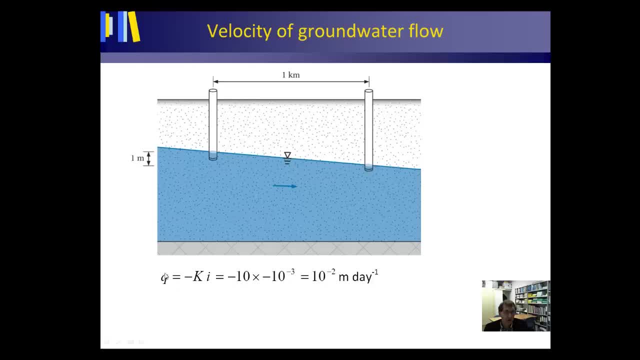 10 to the power minus 2. so if we multiply these two, we get a volume flux density of 10 to the power minus 2 meter per day, which is one centimeter per day. this, of course, is not the velocity. the velocity is your volume flux. 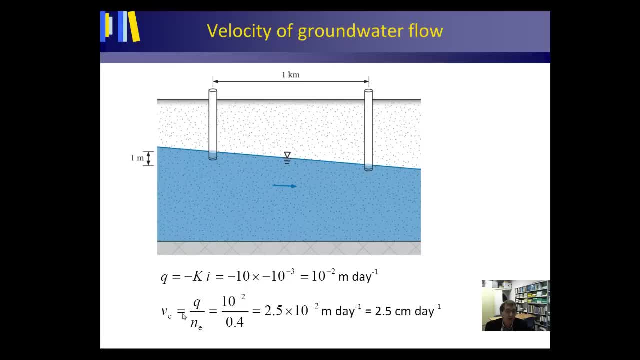 divided by your effective porosity, and an effective porosity of a sandy aquifer can be somewhere in the vicinity of 0.4 if it's well sorted. sand 10 to the power, minus 2 meters per day divided by 0.4, which will give you a velocity. 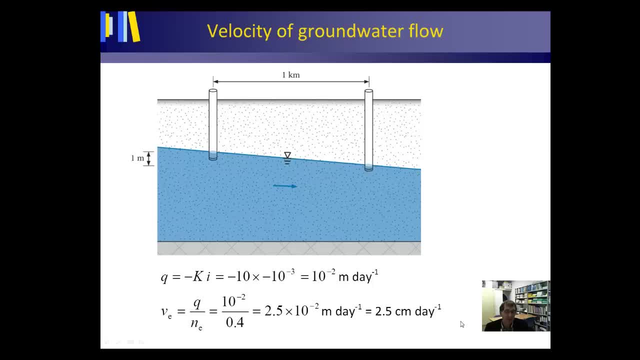 a real velocity of 2.5 centimeters per day. then of course we can also establish what the time is for water to flow from the left piezometer to the right piezometer, and with a velocity of 2.5 centimeters per day.